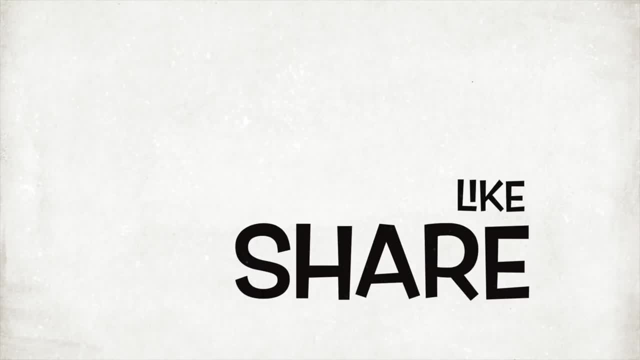 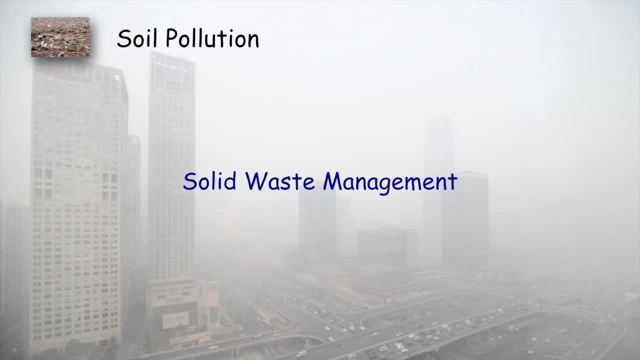 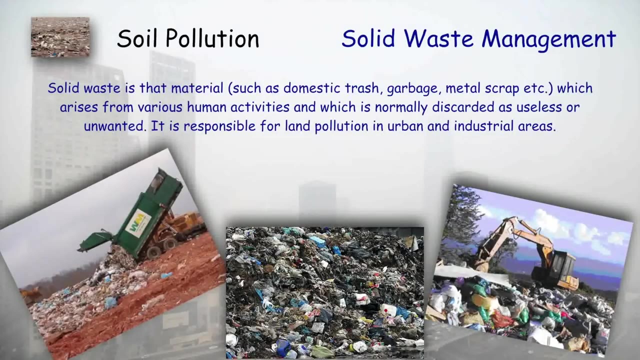 If you like my videos, please click on the like button and share it with your friends. also subscribe for the new videos. So our next topic is solid waste management. Solid waste includes generally. solid waste are the materials which we are throwing from our domestic uses. it includes trash. 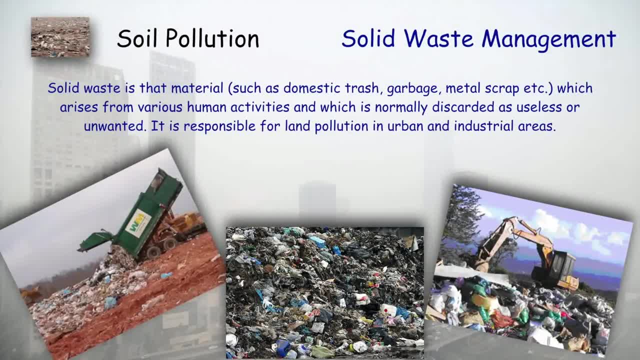 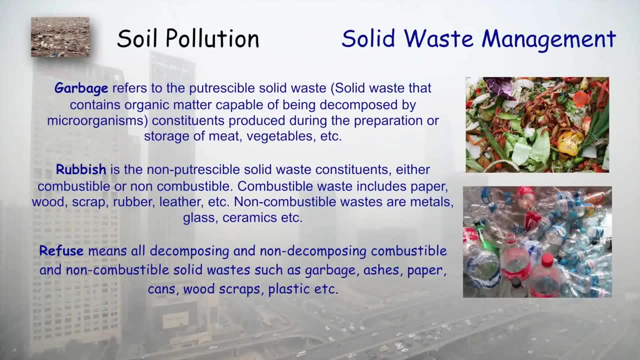 Garbages, metal scraps etc. Which arises from the daily human activities and which is normally discarded as useless or unwanted material. So it is going at to the towards the land pollution in urban as well as industrial areas. There are three terms. one is garbage, rubbish and refuse in case of solid waste management. 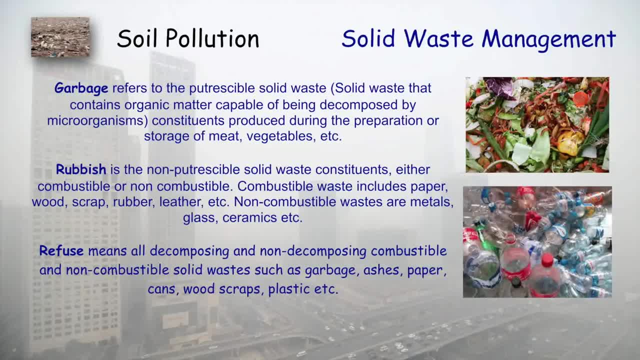 So garbage may refer to the any material, any solid waste which may contains organic matter or contains the biodegradable or decomposable materials. and what about rubbish? rubbish is The material, solid material, solid waste material which may include all the non biodegradable material or non. 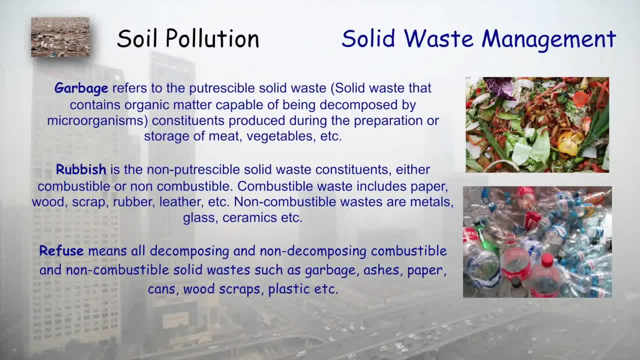 Compostable materials, So for example, like wood rubber, then plastic, then leather paper, etc. and refuse means It means all whatever we have refused to use. so it concludes both decomposing as well as not not Composing material, so it will include both of them, like garbage as well as rubbish. 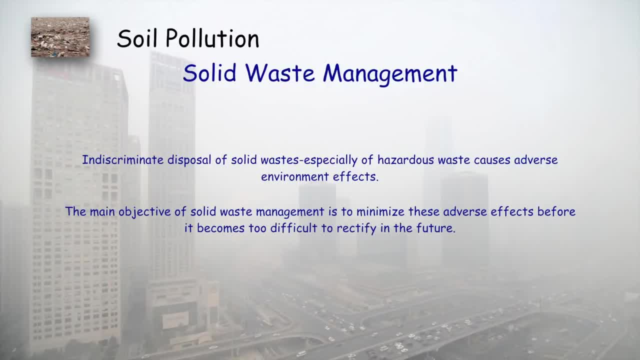 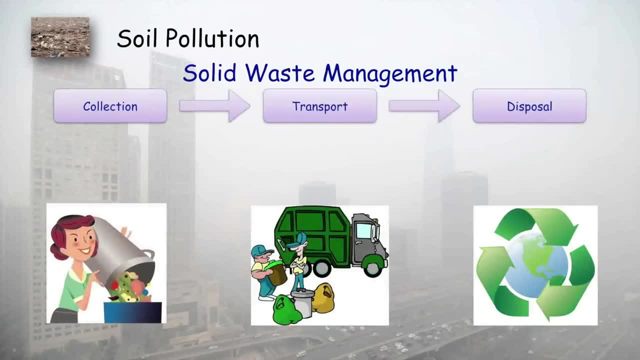 So what is solid waste management? it is the management of the daily waste, daily solid waste discarded from the human beings or Anybody who is not using any of these things, and This includes mainly three steps: one is collection, second is transportation and third is disposal. so, in terms of collection, 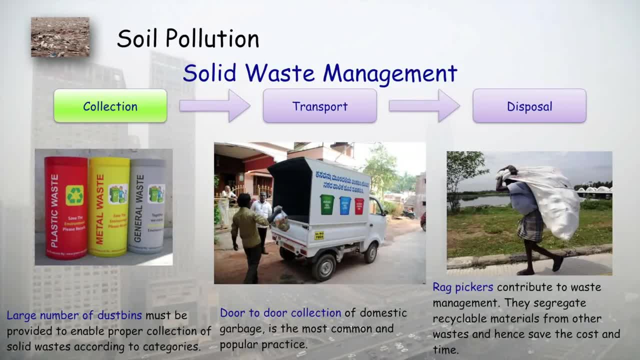 first of all, the ways of collection. There are many ways of collection, collecting solid waste. first is the use of large number of dust winds. We must implant, implant a large number of dust winds all across the city. And then there are some of the door-to-door collection facilities are also available. 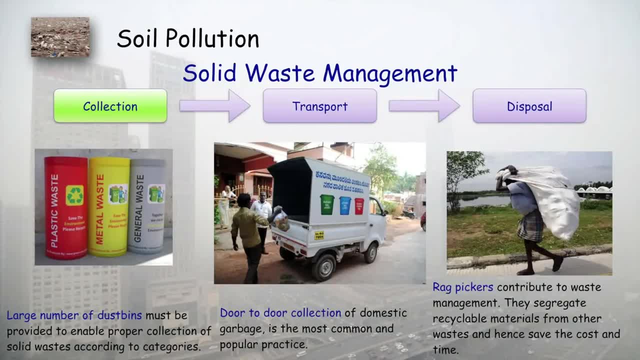 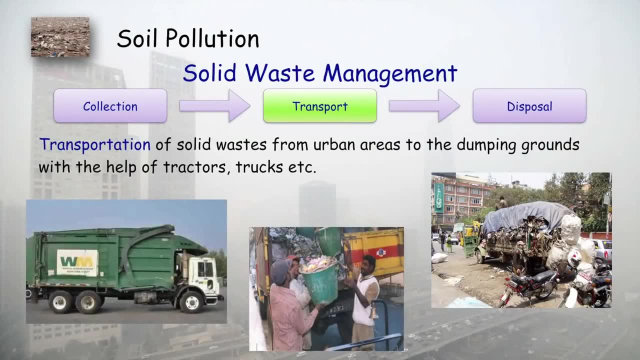 And then, finally, there are some rag pickers, who generally collects the usable material from the, from the dumping grounds and everywhere. What about transportation? for transportation we need highly equipped. And then, finally, it is the use of the large number of the packaging products for the transportation. Then there are many workers who work on these things. 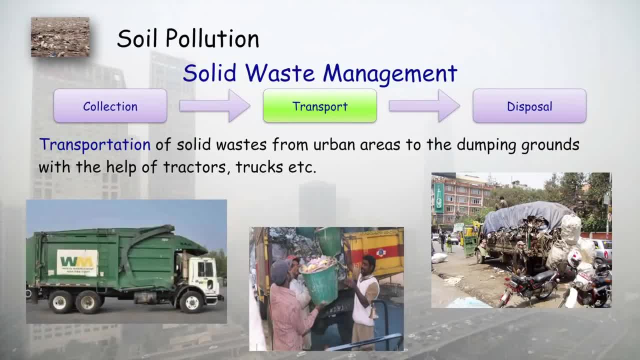 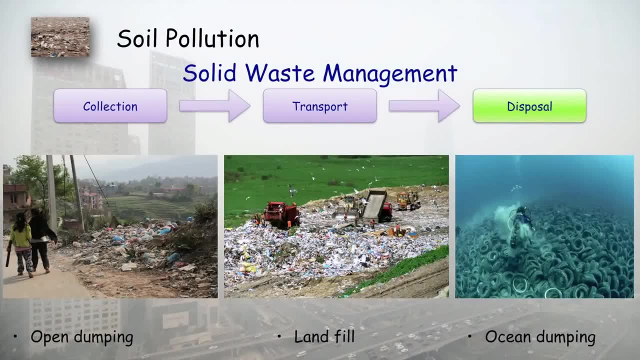 But it is important for the safety of the workers that they should use the hand gloves as well as the mask, because It is a hazardous way of use of doing the work. And finally, disposal. there are several ways of disposing this solid waste management, solid waste, and One of them is open dumping. open dumping means if you find some open place, 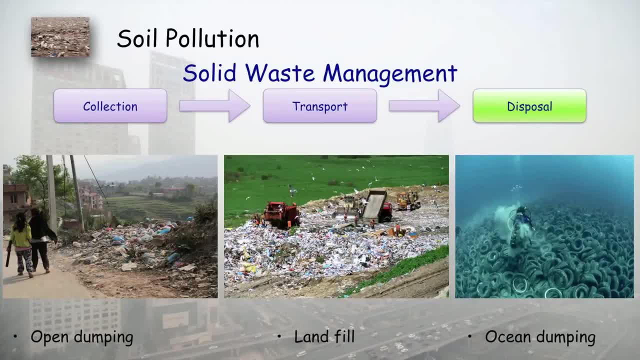 called as the open dumping, which is not really good for the society. then second comes with the landfill. landfill are the areas which are given by the government and where all the garbage from the, from the city is dumped across there. so that is landfill, and the third one is the ocean dumping. 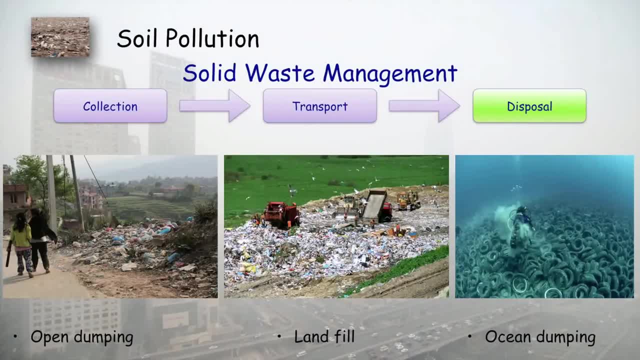 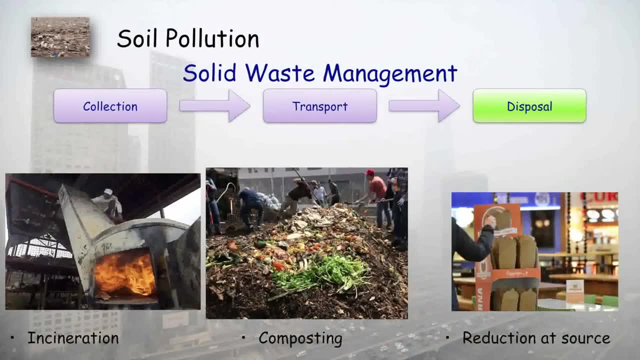 ocean dumping means generally, we pack the materials, pack the solid waste in a proper way and dump it into the ocean, which is also not good because it affects the aquatic life. there are many more ways of reducing the solid waste, so one of them is incineration. 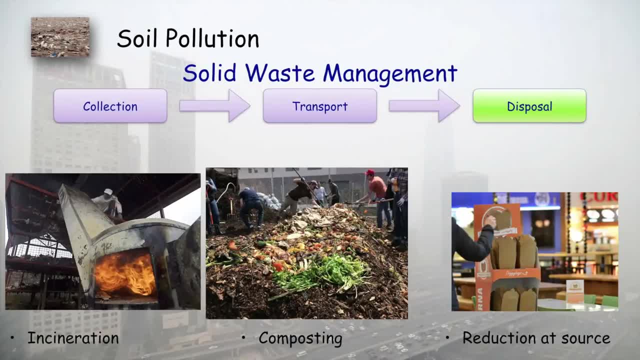 incineration means we can burn the solid waste and then we can produce energy or heat out of that, but it also produces the carbon dioxide as a pollutant over there. next is composting. composting means all the biodegradable materials can be converted into compost. 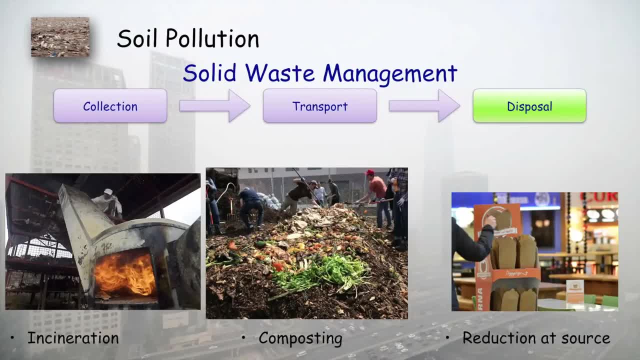 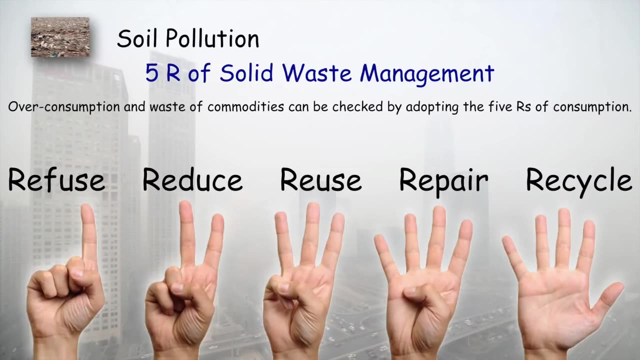 which can be used as a fertilizers in agriculture and anywhere. and the last one is reduction at source. reduction at source, that means we should reduce the making of solid waste, so it should not be generated too much. we should not generate too much of the solid waste. next is five are of the solid 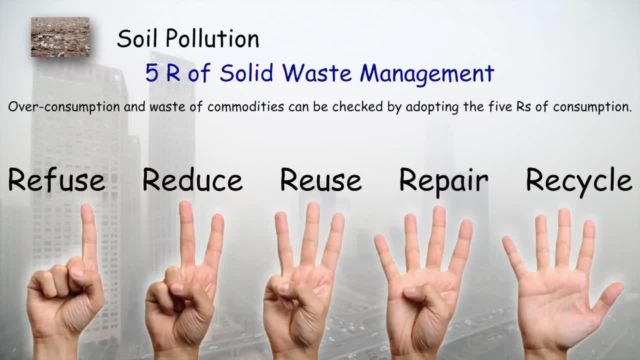 waste management, and these are: refuse, reduce, reuse, repair and recycle. so first of all, we need to refuse the uses of non-biodegradable materials, then, if it is necessary, we must reduce the uses, and if and if there is still some uses, then we we must go for the reusing. same thing again and again.